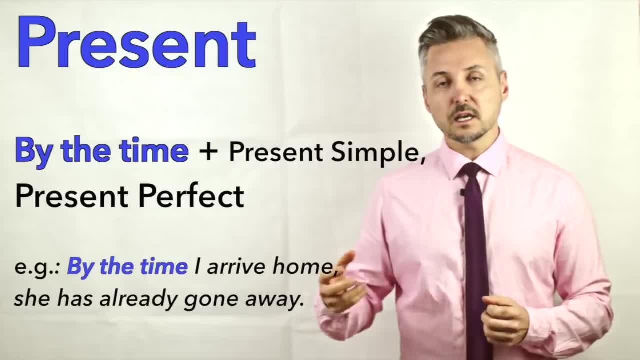 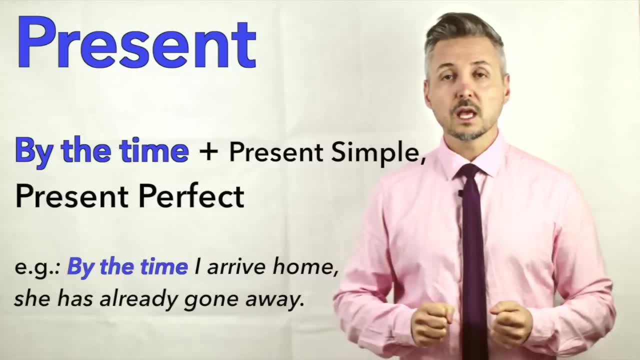 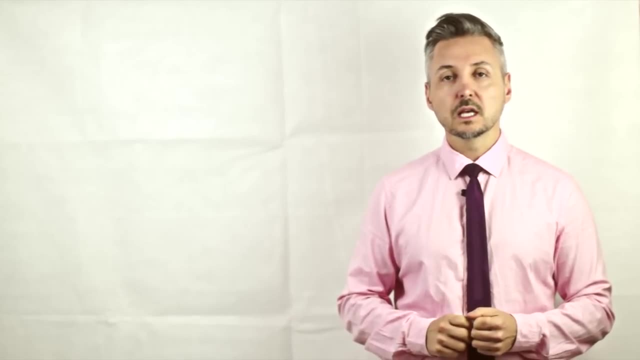 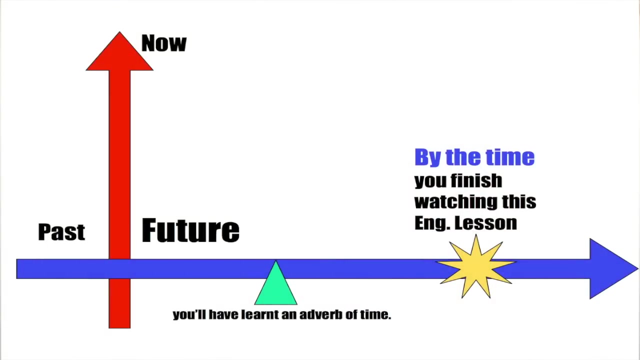 plus present, simple, and then the present perfect. So by the time I arrive home she has already gone away. Now let's look at by the time. in a timeline You can see that the first part of the sentence is the second part of the timeline because something came before by the time. So the example that I gave 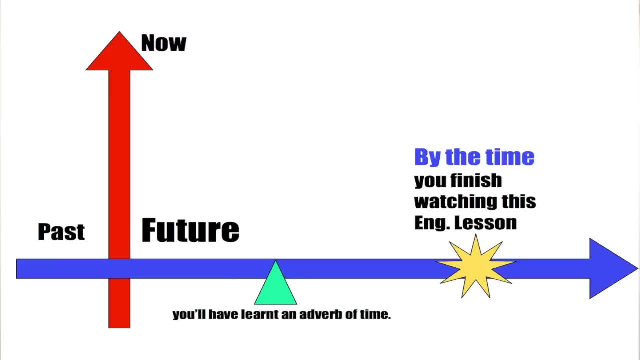 you was. by the time you finish watching this video or this English lesson, you will have learned it from here By the time…. So this is the first section like this one By the time, that which was before and is an adverb of time. An adverb of time is the first action that 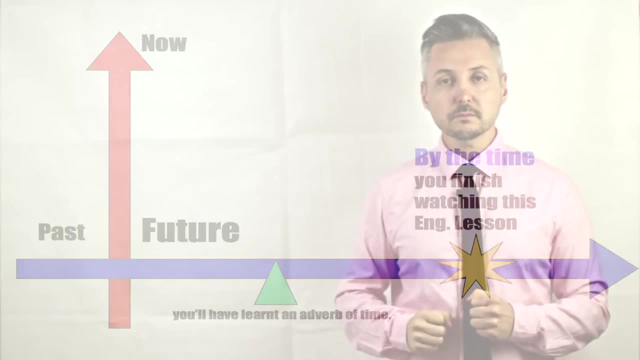 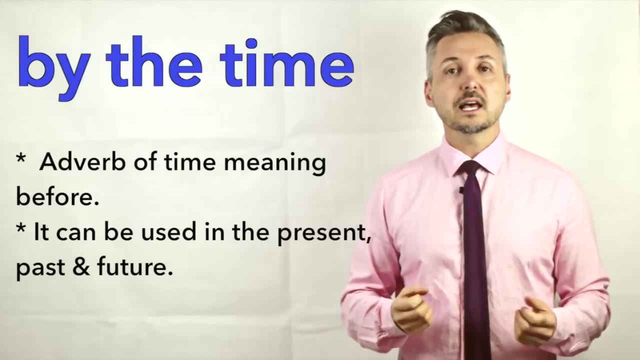 happened in the timeline and then finish the video. the English video is the second action that you will see in the timeline: An adverb of time. Now let's recap. I said by the time means before and is an adverb of time. We use it in the present, in the past. 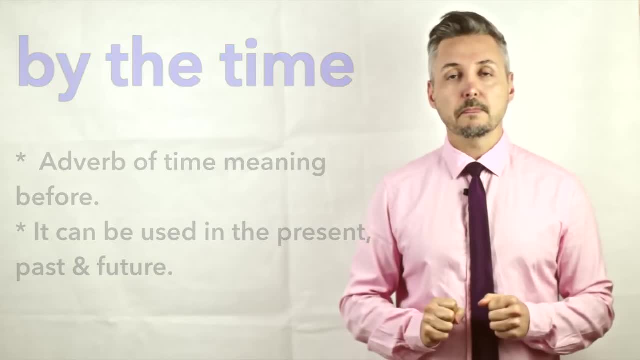 Let's off the內ers. Let's bring the say-ins for the next one that was asked for just before. by the time. Let's bring the say-ins for the next one that was asked before. by the time past and in the future, You have to pay attention to the different types of formulas that we use. 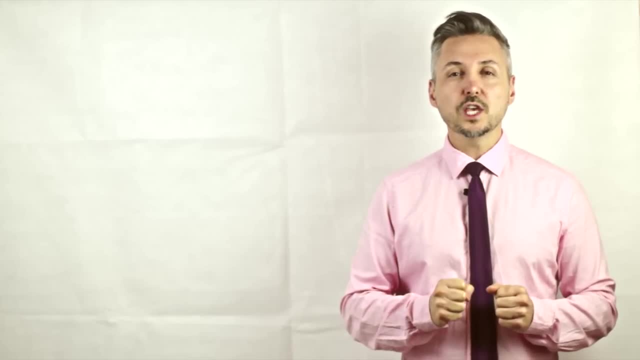 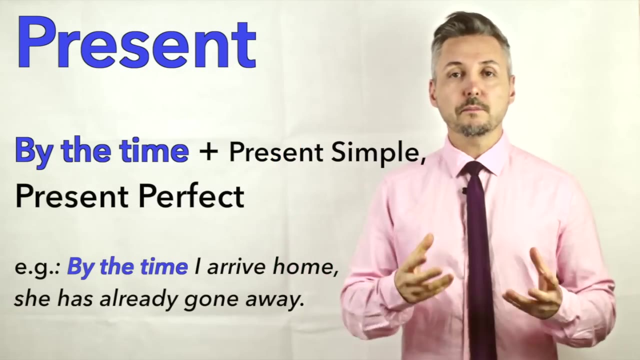 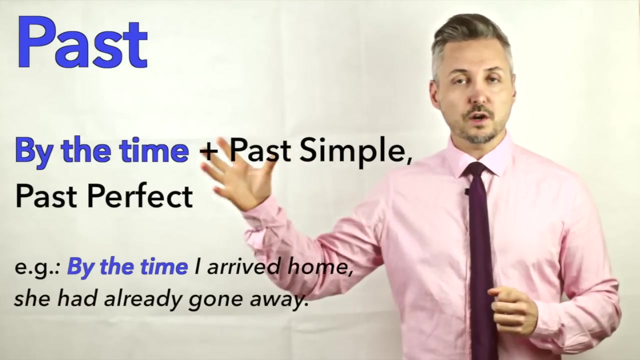 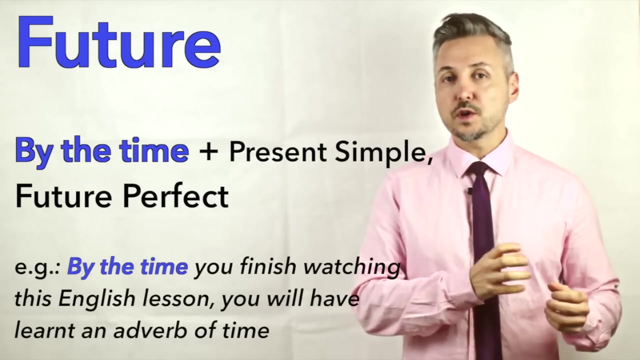 with different tenses. So for the present we use by the time plus present simple and the main clause we use the present perfect. For the past action we use by the time plus the past simple and then the past perfect in the second clause, in the main clause. And for a future action we use by the time. 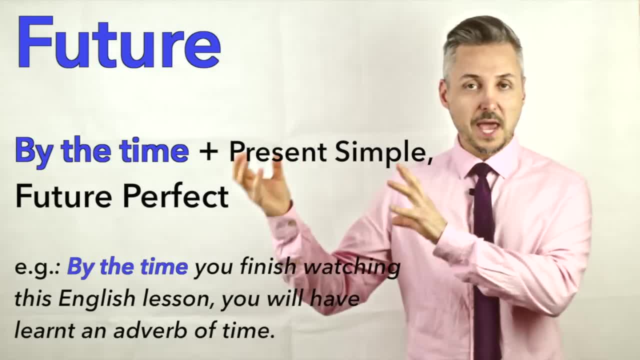 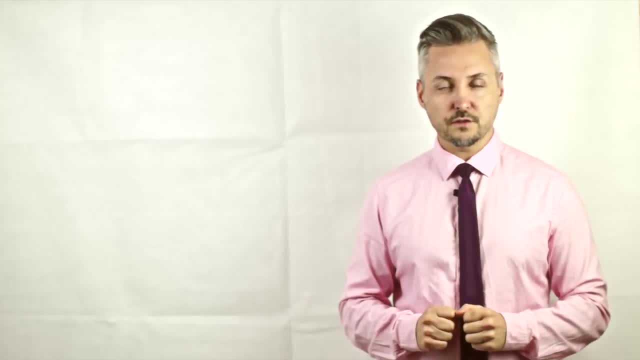 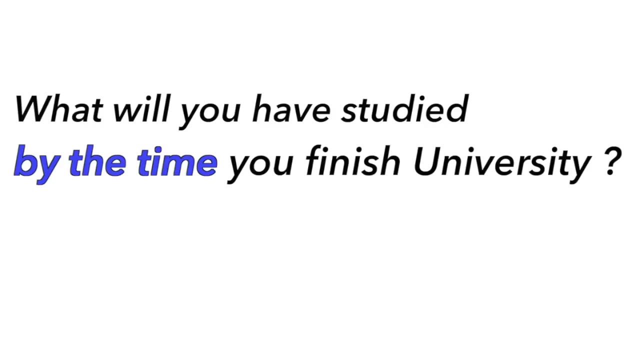 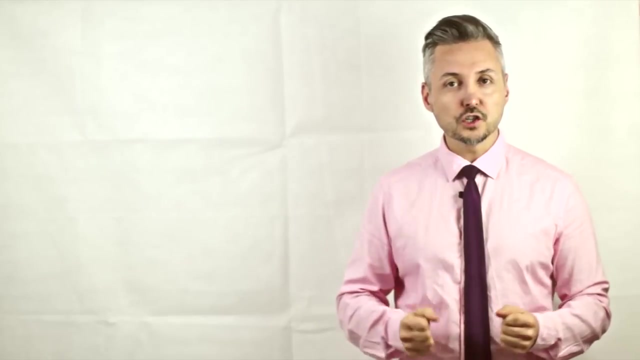 plus, the present, simple plus. in the main clause we use the future perfect. So now I have a question for you: What will you have studied by the time you finish university? What will you have studied by the time you finish? So have a nice day. I hope you enjoyed this video. Please share it and I see you next time. Take care, Bye, bye.